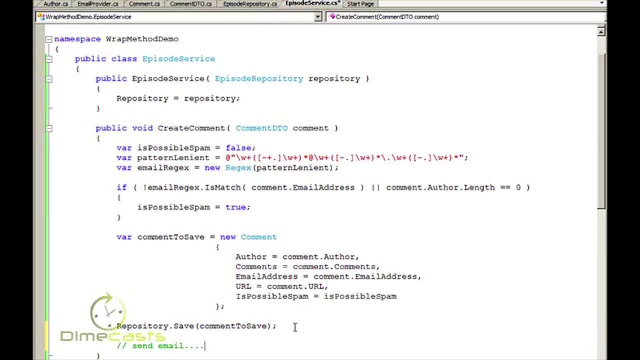 but that's a problem, because what you're doing is you're adding complexity to this method. You're decreasing the refactorability in the future. You're also just adding responsibility to what the create comment method is meant to do, Because, up above everything, this is all. 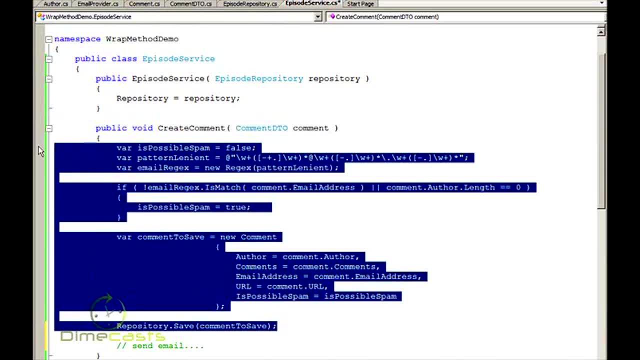 about one responsibility: creating the ability to save a comment. Sending an email is a completely new responsibility. So what we want to do today is look at the ability to save a comment. So what we want to do today is look at the ability to save a comment. So what we want to do today is look at. 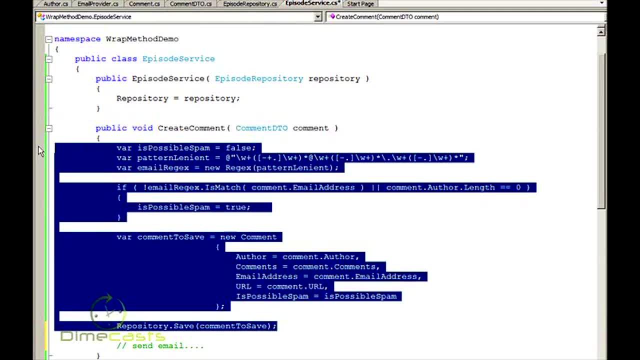 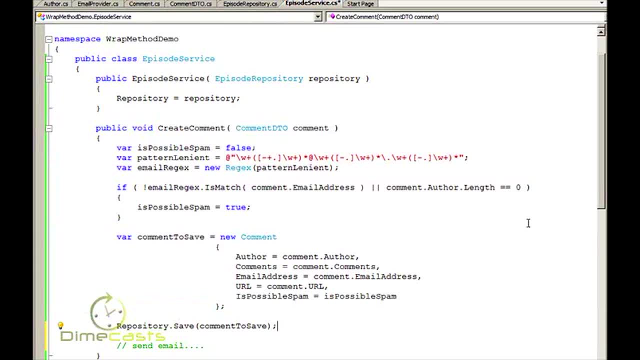 the wrap technique that will allow us to you know more simply add this functionality and do it in a safer, more maintainable way. Now the first thing we want to do when starting this refactor and to create the wrap method is: I want to take all this code and I want to move it out of the 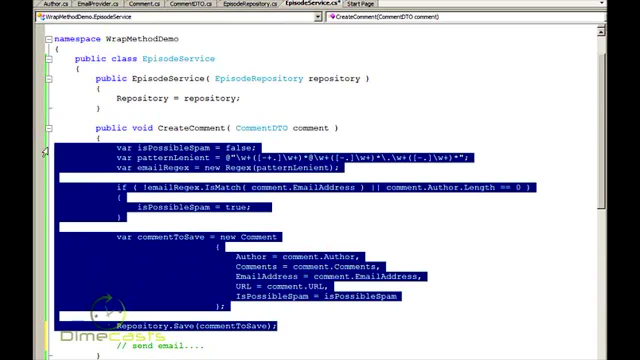 create comment, And the reason for that is the create comment will now have two responsibilities and I want to make sure that I can segment my two responsibilities at least in two separate methods internal to my class. So let's go ahead and do the extract method And we'll call this. 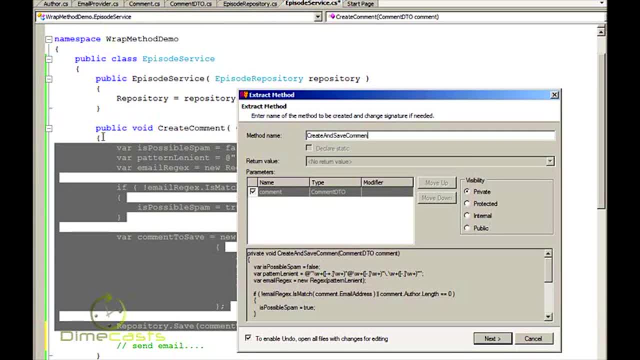 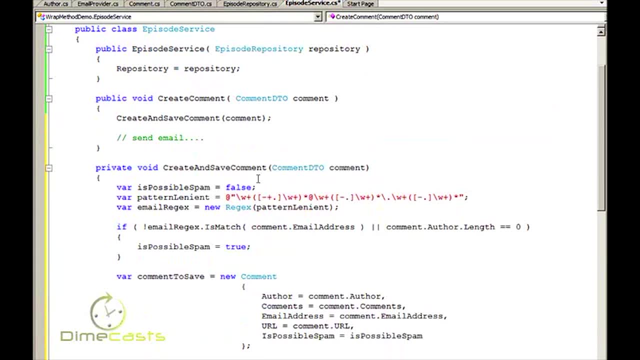 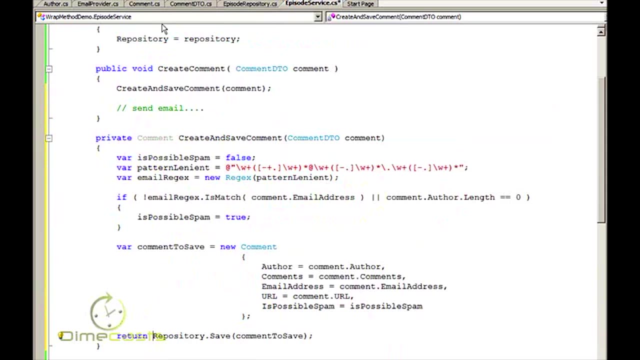 create and save comment And the create and save comment will take in our DTO and it will basically just perform all the logic. Now I want to do one extra thing here. I want this to return my comment. So we now have refactored this so that it is a separate method and create comment just calls that. 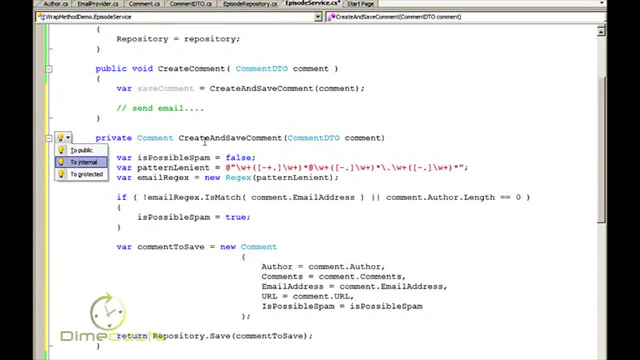 method. Now I would like to go one step further. What I also want to do is make this protected virtual, because by making this protected virtual, I can, you know, do another testing technique where I create a- you know, a stub of this and I can actually test this method standalone to the public. 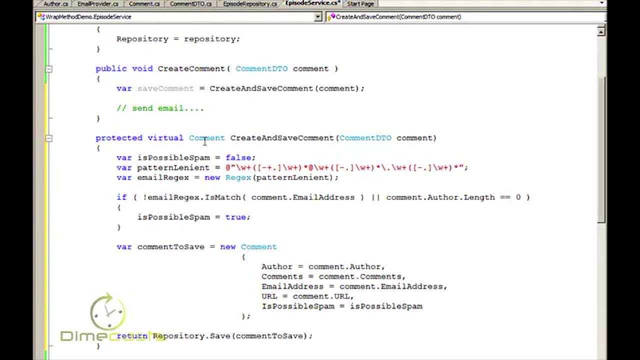 method that it's calling it. Now, I understand that, making things virtual, it does have a slight performance hit and does open up for later extensions for people if you don't want, but that's a choice I choose to make. Now the wrap technique comes in, where I'm going to create now a 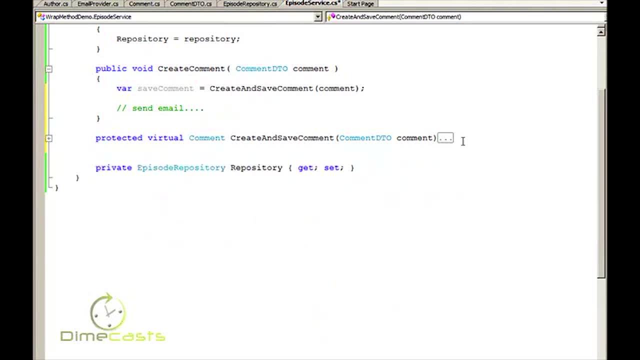 second method here We'll call this protected virtual send email to author And this will take our comment And I can now come up here and send the email to author, save comment. So what I've effectively done is I've taken this new functionality. 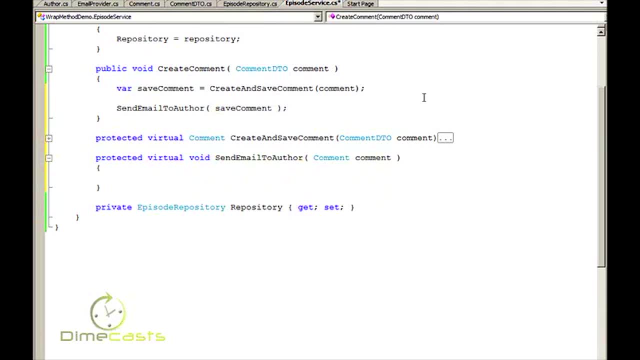 I've extracted it from the original location, I've moved it into its new method and would go- wouldn't go a couple steps further here in a second. But now I basically set it up so that my create comment just wraps all the various things that it needs to do. But it really is only calling. 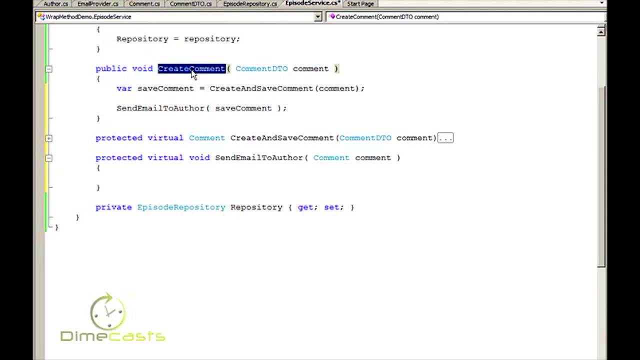 it off into other methods, And these other methods could be in other objects, They could be other namespaces, They could be anywhere you want, But this create comment just wraps them. for us Now to go ahead and fill this out. what I'd want to do is do something like this: 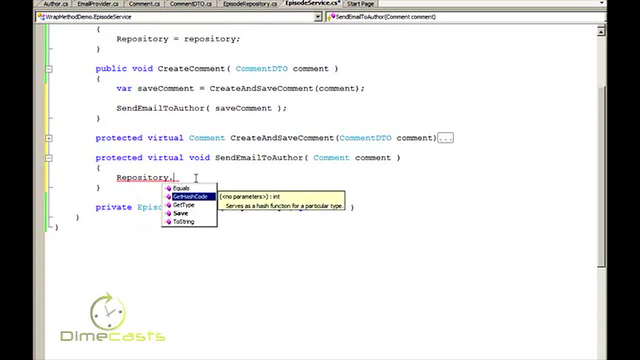 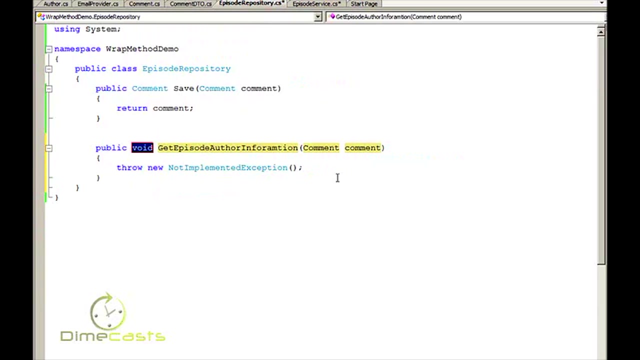 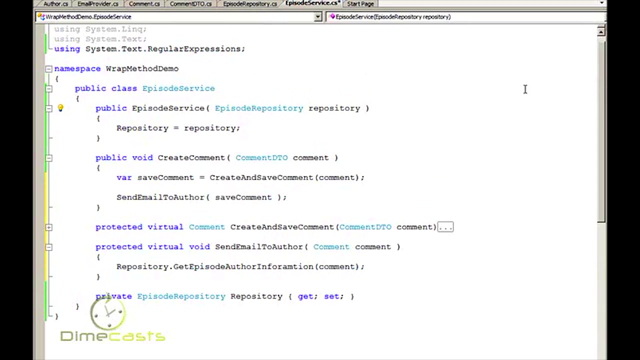 Repository And I'd want to do something like get episode author, You know, call into some method to get the episode author information And we'll go ahead and create this And we'll just fill this out real, real briefly. And I've already got a email provider, So email. 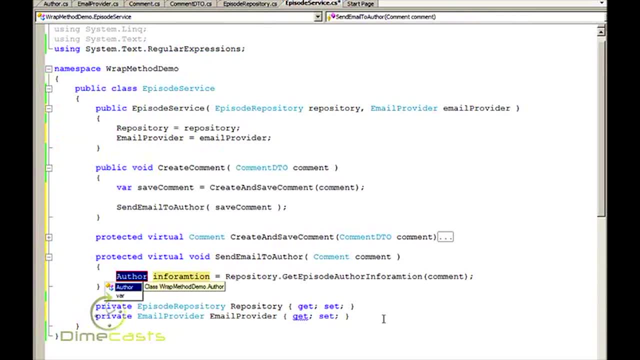 We won't actually fill this out. We don't really care because the intent of this is to explain the refactor technique of wrap method. So if we step back to the original, intent of this is to extend the create comment logic and concept to not only save the comment but, once it's done saving, send an email to the author. 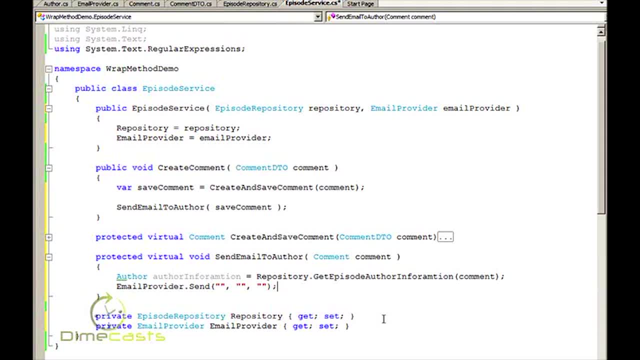 And by utilizing the wrap refactor method- wrap method, refactor method- instead of adding all that logic into one big method where it would be very difficult to test individual pieces. I just added: I segmented each of those responsibilities into their own methods, which would now allow me to actually test each one of them individually.